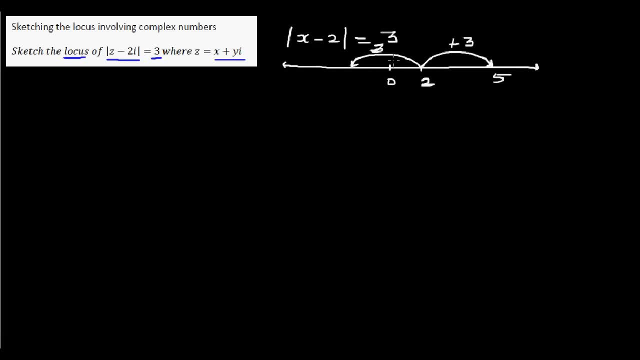 3 to the left. So 3 take away 2.. So this is minus, so negative: 1.. So when you solve this, so modulus of So this is how we do it algebraically. So when you solve this, so modulus of So this is how we do it algebraically. So when you solve this, 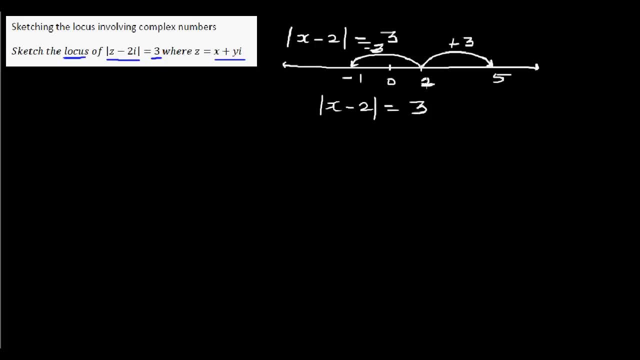 so z minus 2 is equal to 3.. So basically, this is the idea of modulus. So the two numbers which are at a distance of 3 from 2 are 5 and negative 1.. So how do you do it algebraically? So well, we can say: 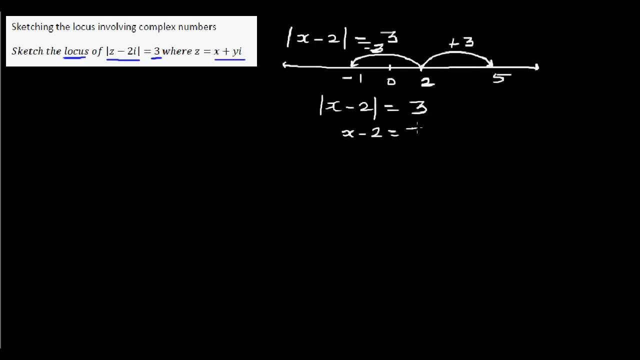 x minus 2 is equal to 3.. That's one option. Or x minus 2 is equal to negative 3. Because modulus can be positive or negative. So adding 2 to both sides x is equal to 5, and adding 2 to both side x is equal to negative 1.. 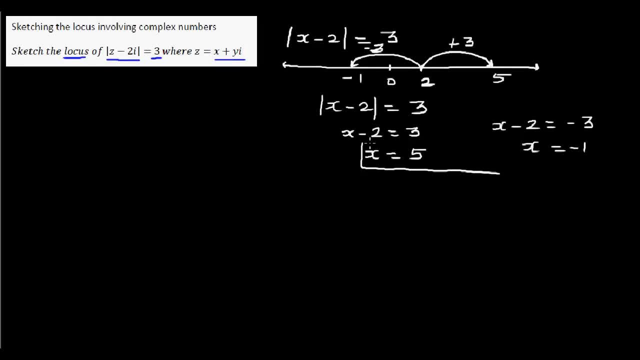 So this is the algebra and this is the graph. So the Idiom complex number is basically the same, but as it's complex number, you have to think in a slightly different way. So what does this mean? So let's understand this. Modulus of z minus 2i is equal to 3.. So basically, 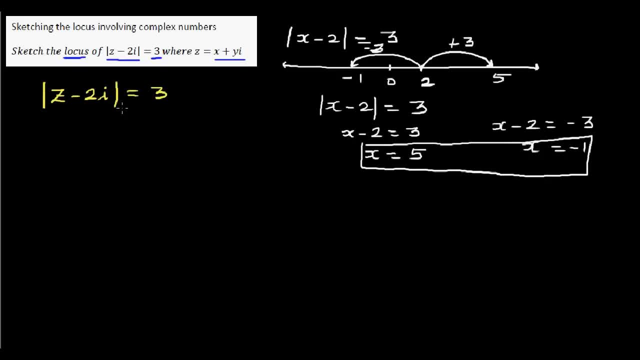 we're asking? we're asking for the sum of the problems sized all the way to the total values. the question tell me the complex numbers which are at a distance of 3 from 2i, so let's graph this. so what does this mean? so where is 2i? say this, is, this is. 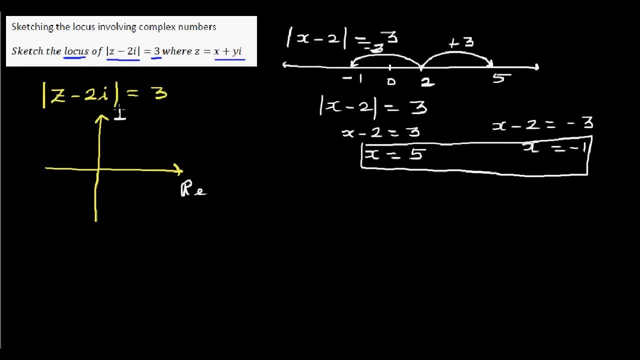 your. this is the real arm and this is the imaginary arm. so the same idea: z minus 2i, so 2i is somewhere here. so this is 2i. so tell me all the complex number which are at a distance of 3. well, it is basically a circle. so 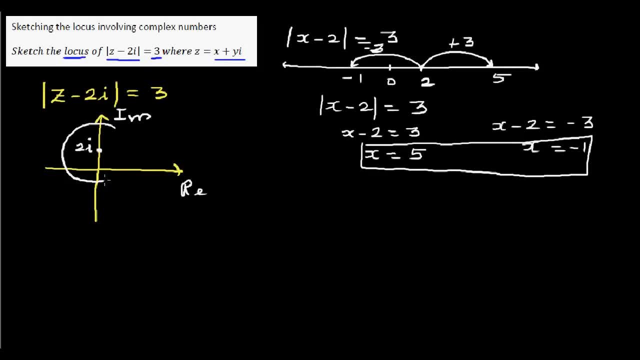 let me draw a circle somewhat, looking like this: so all these, so this is at a distance of 3, so this is the radius of 3, so this is also radius of 3, so this is basically a circle. so here the locus is the set of all the points which are at a 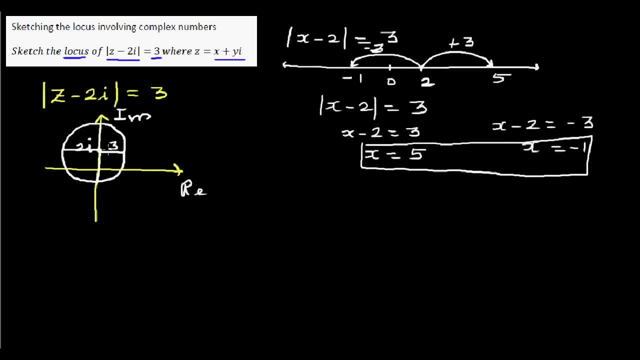 distance of 3 from the center, which is a 2i. so basically, just looking at this question, I can say this is a circle with center 0, comma 2i and a radius of 3, and if you want to write this algebraically, this is: x squared plus y minus 2, the whole squared is equal to 9. but let's do. 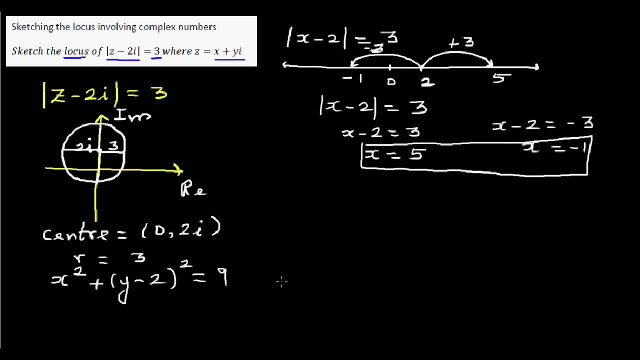 this algebraically? how would you get this answer? so so the question is: modulus of z minus 2i is equal to 3, so by just looking at this question you can tell the answer: all the set of points which are at a distance of 3 from this. 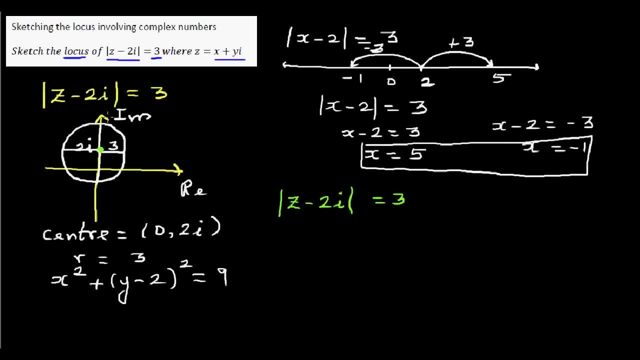 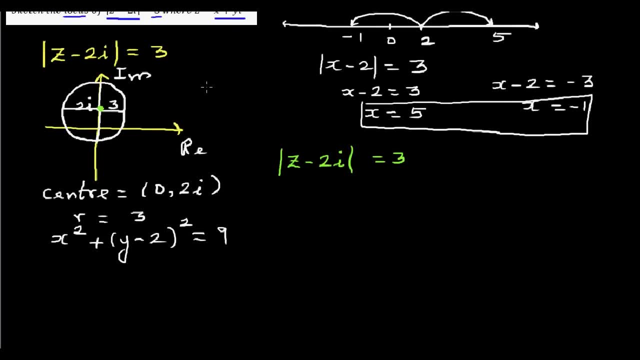 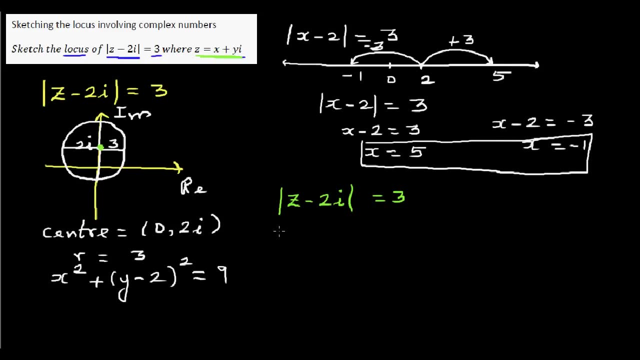 center, which is 0 comma. 2i is the complex or is the locus, so writing this in a z where z is said to be, where z is said to be, x plus yi. so in place of z I can put x plus yi, so this changes to x plus yi. minus 2i is equal to 3, so 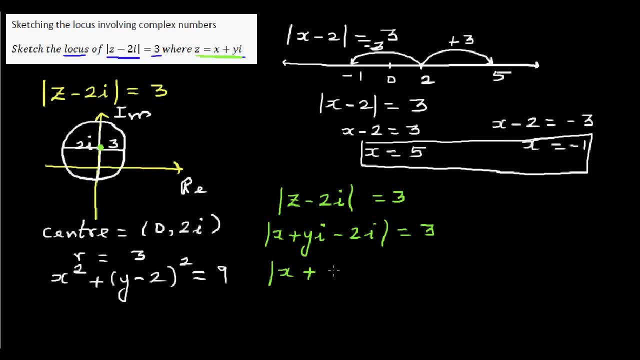 writing this in rectangular form, it is x plus taking the i's out, y minus 1, this should be 1 year. I made a mistake here. okay, Y minus 1, y minus 2. sorry, and it's not. this is: if you take the I out, 2 is equal to 3. so this is right, because if 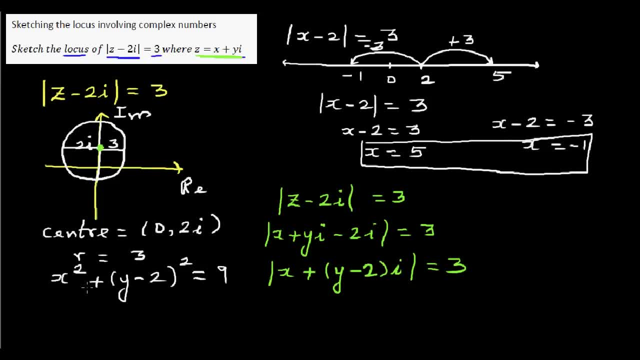 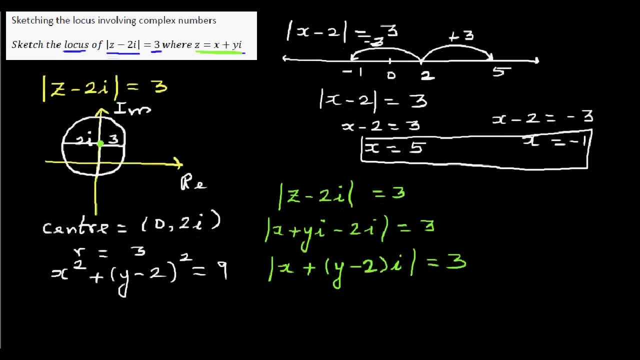 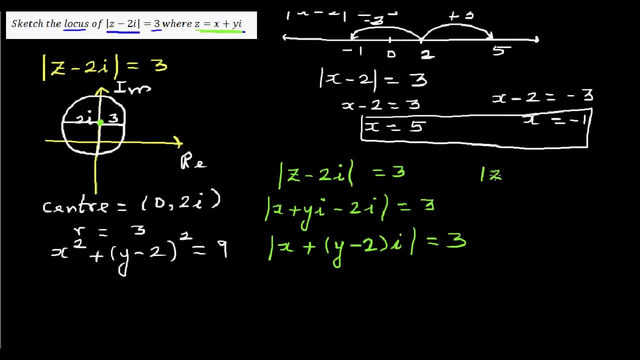 this is center 0 comma 2i, and so the center is 0 comma 2i. so this is X plus y minus 2. okay, so what does this mean algebraically? so this means, if you write this, the formula of modulus of Z is x square root of x squared plus y. 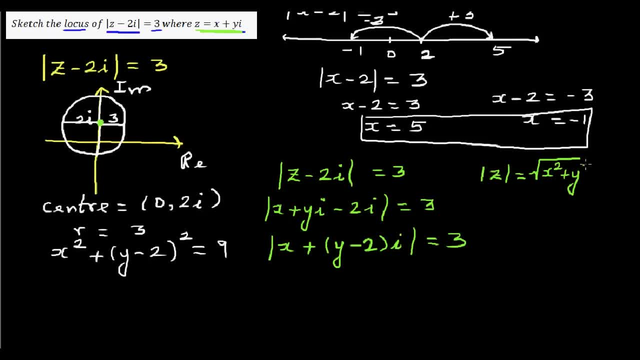 squared, modulus of Z is square root of x squared plus y squared. so modulus of Z is square root of x squared plus y minus 2. the whole squared is equal to 3 and if you square both sides, this is x squared plus y minus 2, the whole squared. 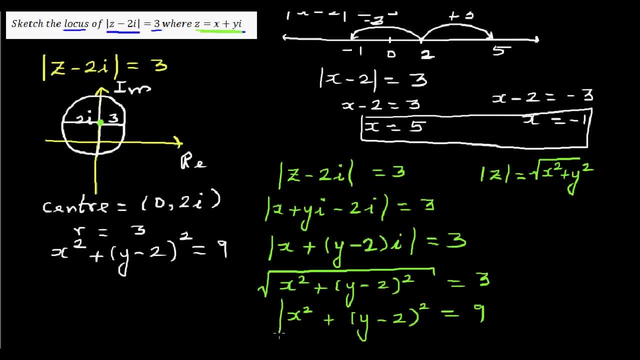 is equal to 9 and that's what we got. so this is the locus and if you want to draw, want to go backwards, this has a centre of and a radius of 3.. I hope you know. the equation of a circle is x minus a whole squared plus y minus. 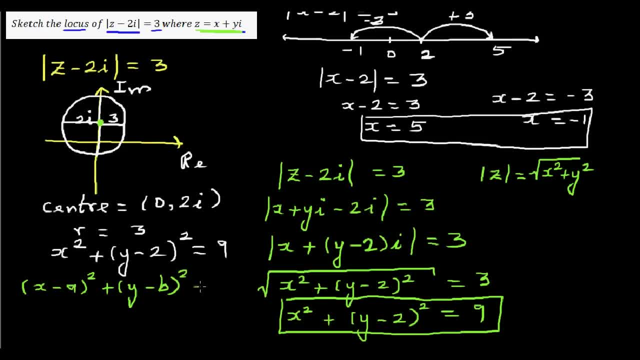 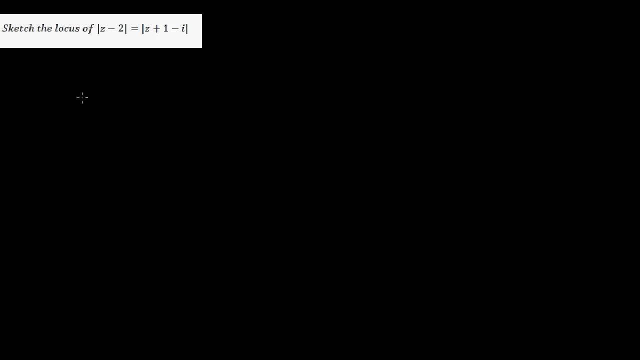 b, the whole squared is equal to r squared where centre is and radius is r. Okay, so let's look at one more question Sketch: the locus of modulus of z minus 2 i is equal to modulus of z plus 1 minus i. So let's first do it algebraically. 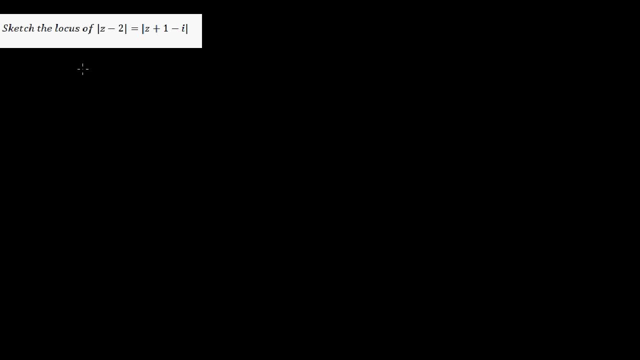 without doing that, sorry, graphically, and then we will do it algebraically. So let's understand. what does this mean? z minus 2 is z minus 2.. So here we are asking the question, the complex number at a distance. 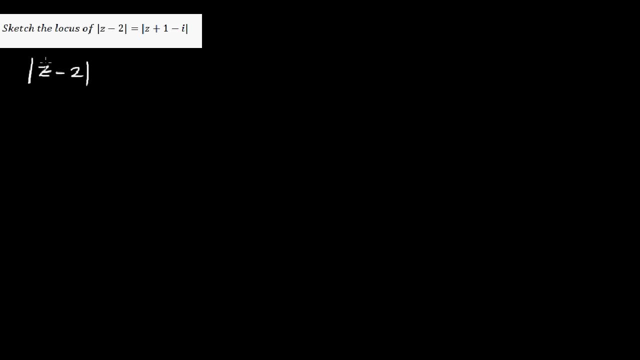 distance of 2.. Okay, so all complex numbers at a distance. sorry, the distance of z from 2 is equal to the distance of writing this. in this form I can say this is z. I'll put a minus out. so can you write this as negative: 1 plus i. 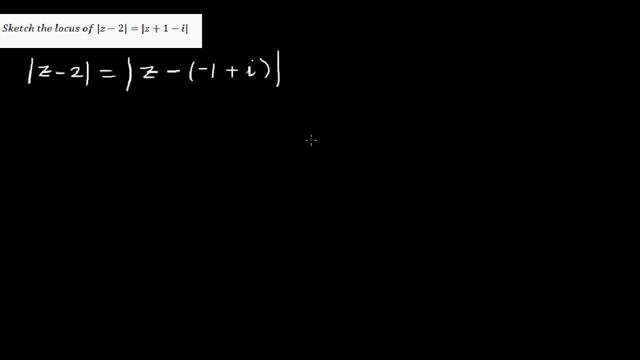 This is the trick part. So basically, if you want to, what we're saying is a set of numbers which are at the same distance from these two conditions. so let me explain this. so let us graph this: So z minus 2, so basically, this is so modulus of z minus 2 means. so this is: 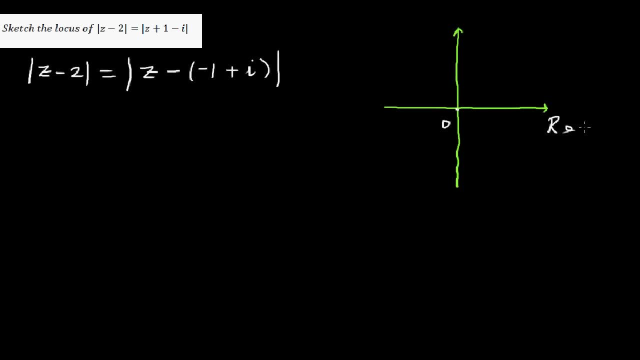 zero. this is the real arm and this is the imaginary arm and a term which known as Edward Cresden. okay, so 2 comes here. so this point is 2, or this is 0, 2 and this is minus 1 plus i, so this is minus 1. 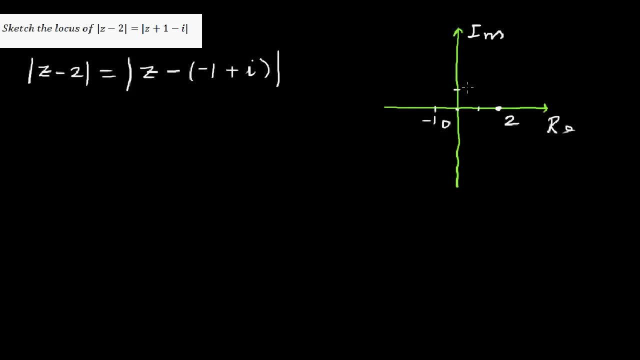 and this is plus i, this is i. so this point, this point, is minus 1 plus i. so basically, you're thinking of all the points which are at an equal distance from these two points. well, that is going to be a straight line, okay. so you can think of: if you have two points, you can get a set of points. 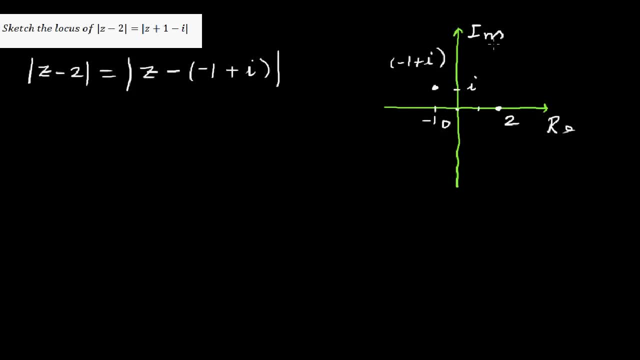 which are at the same distance. so I know the answer. we'll have to prove it. so the line would look somewhat like this: okay, so this line is at the same distance from these two, these two complex numbers. okay, so this distance is equal to this distance. so, basically, the answer. 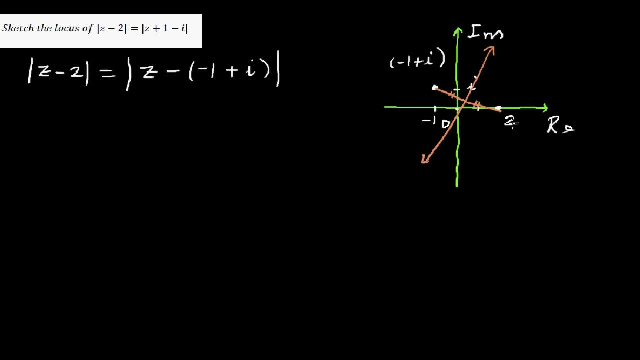 of this question is a straight line and all these points. if you take any arbitrary point, say if you take this point here, let me use a different color or green. if you take this point or any point, say this is point x. if you join it, join to this point and this point. 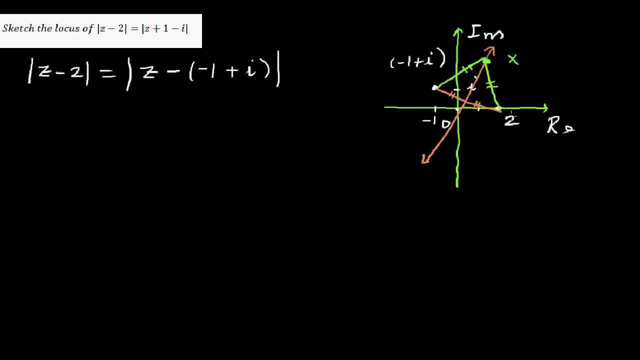 they are equal. so basically, the answer we know should be a straight line. so what does this mean? so writing this, so this basically means this is x plus yi minus 2, this is equal to x plus yi plus minus i, so this is modulus of x minus 2, writing this in rectangular form: plus yi is equal to: 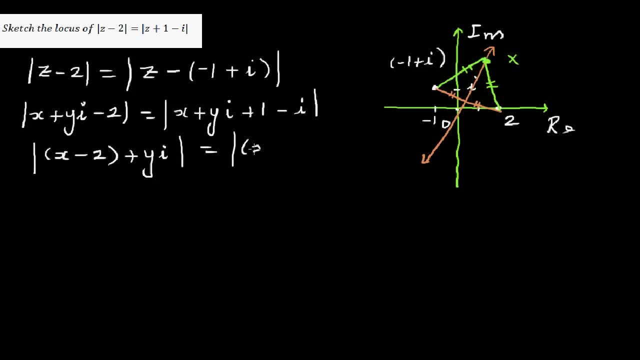 modulus of writing this in rectangular form it'll be x plus 1 plus y minus 1i. am I right? hopefully I'm just rearranging, taking the real part, x plus 1, and the imaginary part. if you factor out i, it'll be y minus 1,. 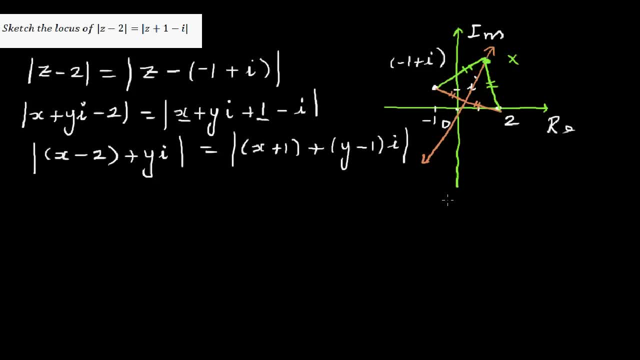 so, as we did, let me repeat: so: modulus of z, if z is equal to x plus yi. this is the formula. this is not the formula. so, basically, this is Pythagoras: absolute value of z would be square root of x squared plus y squared. so, using this same principle, I can say: 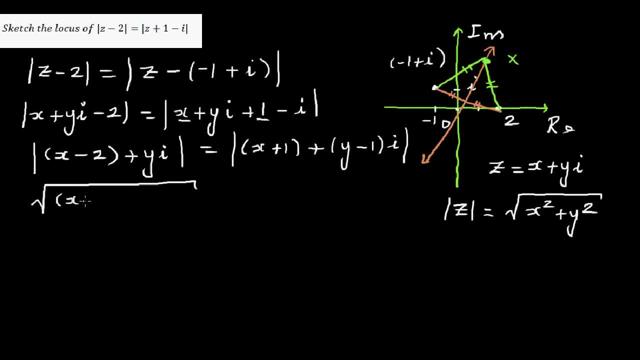 square root of x minus 2, the whole squared plus y squared is equal to absolute value of. sorry. square root of x plus 1, the whole squared, plus y minus 1, the whole squared, So you can square both sides, so this will become x minus 2. the whole squared plus y squared is equal. 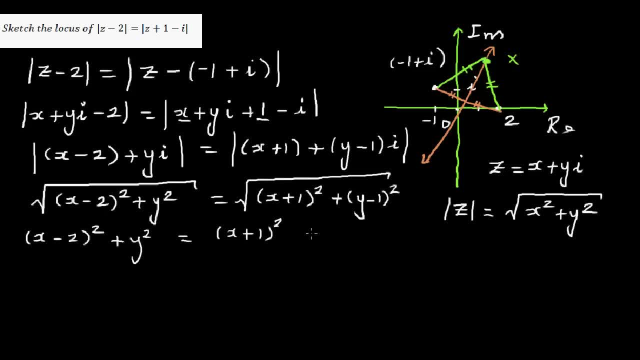 to absolute value of the whole squared. so as I have is equal to ah square root of x plus y. then I would square both sides: x plus 1 the whole squared, plus y minus 1 the whole squared. So, expanding this side, this would be x squared minus 4x plus 4, plus y squared is equal to: 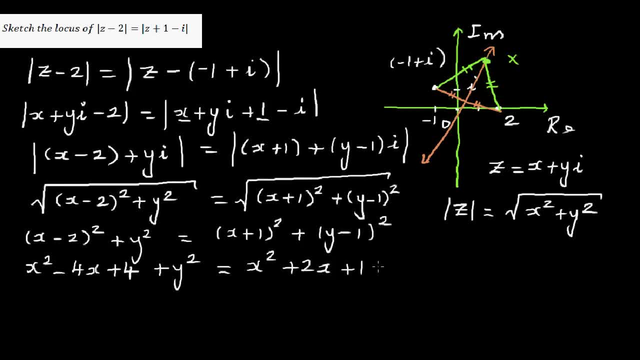 x squared plus 2x plus 1, plus y squared, Ah Ah, Positive minus 4x, negative, 4x squared minus 2y plus 1. okay, so what will happen now? so this plus x squared and plus x squared plus y squared, plus x squared plus y squared, will get: 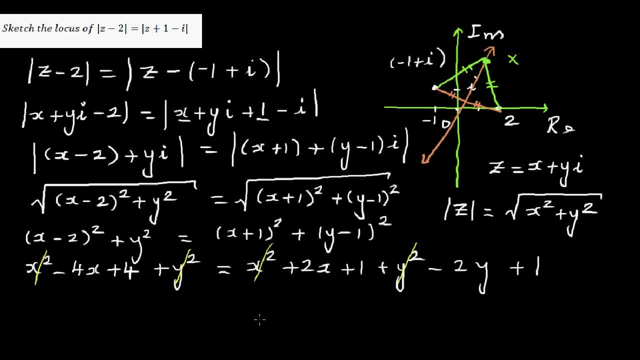 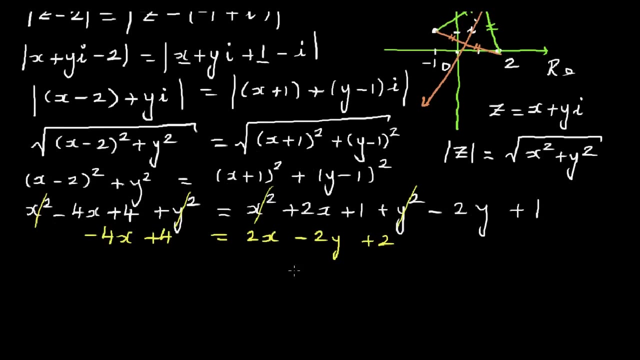 cancelled. so what are we getting? okay, so let's write this. writing this: so what is left out? so minus 4x plus 4 on the left hand side is equal to 2x minus 2y plus 2. okay, so we're almost there, so let's write this as so. let us write: so this is: 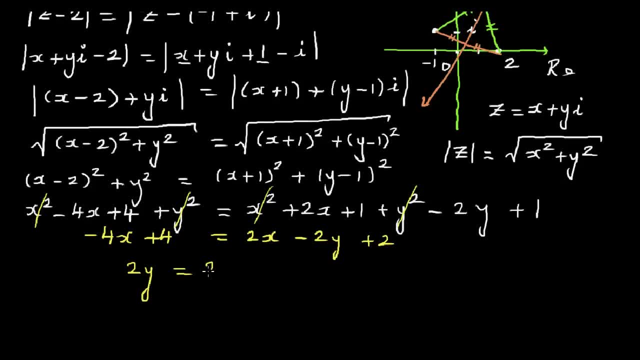 2y is equal to 2x plus 4x plus 2x minus 4. I'm just simplifying. so this is. this implies 2y is equal to 6x minus 2 and dividing both sides by 2, so y is equal to 3x minus 1. so this is basically. 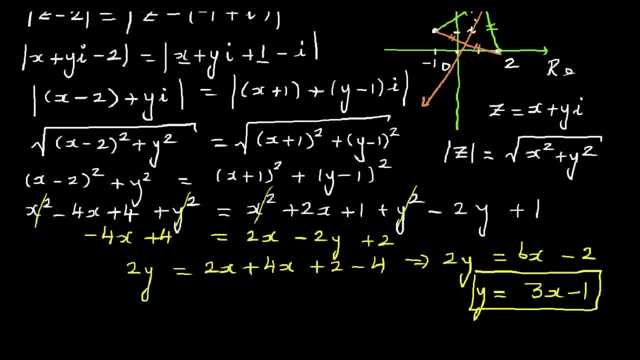 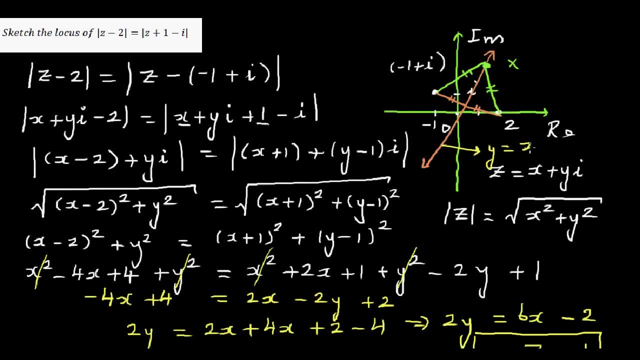 a line. okay, so this line is what I was talking about, this. the equation of this line is: y is equal to 3x minus 1. so if you take any points of this is say: let me explain that this is minus 1 because the y-intercept is negative 1. so if you take that, this distance, this, 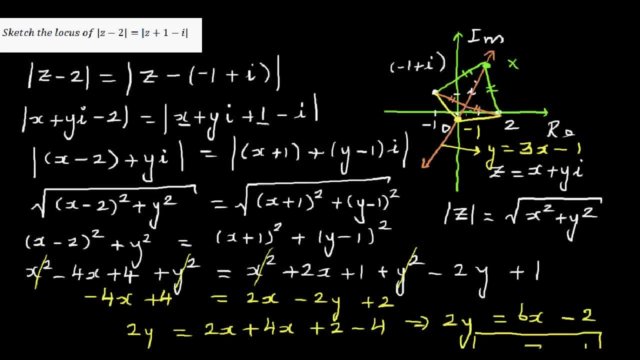 distance is going to be equal to this distance. so if you use 5th Hagris- I hope you understand this is the right. this is you can use 5th Hagris, or this is the rise. you can not just be sorry if you go rise, if you take the rise and run and 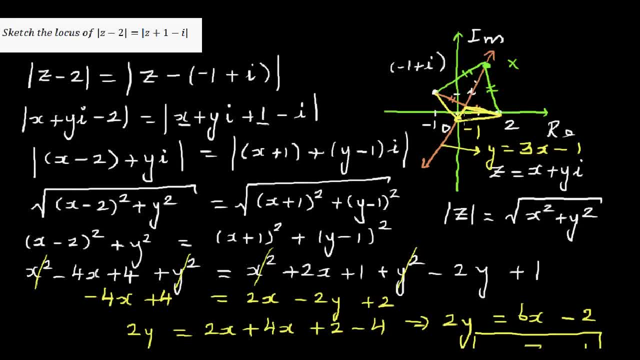 the rise is 1 and the run is full. sorry, at rise is 1 and the run is 2, so this distance is square root of five. okay, the distance from this point to this point is square root of 5. the distance between this point to this point is also square root of 5, so same. 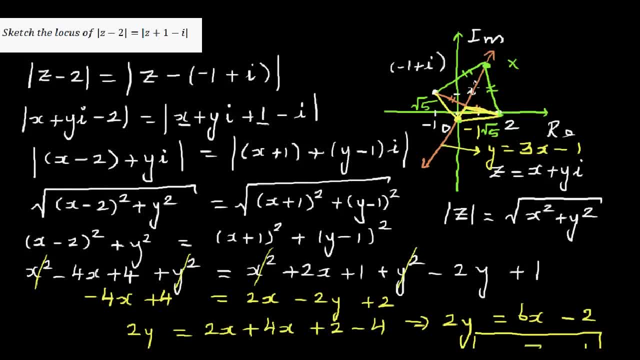 way we can take any point on this and try to find, using the distance formula, the distance between any point on this line, and the nice thing is that the distance gives us δεν is. these two points will always be the same. That is always going to be a constant. 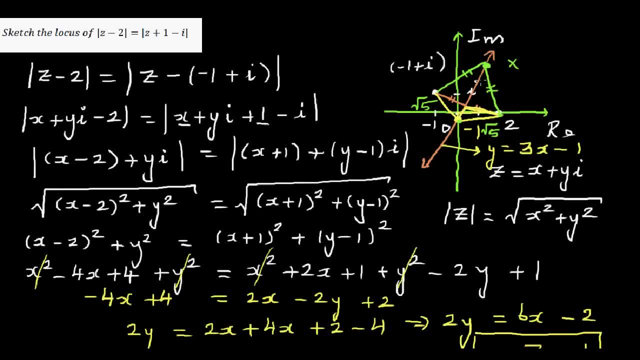 not a constant number. the distance will keep changing, but the distance is going to be constant.